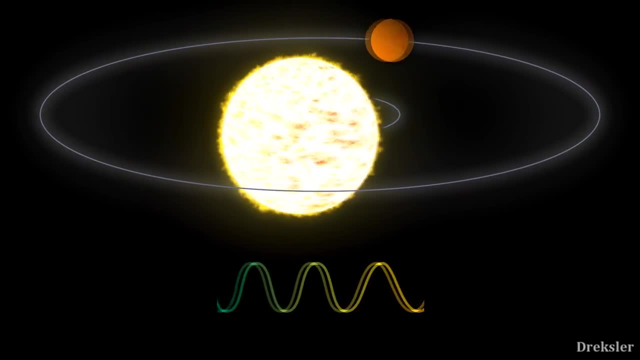 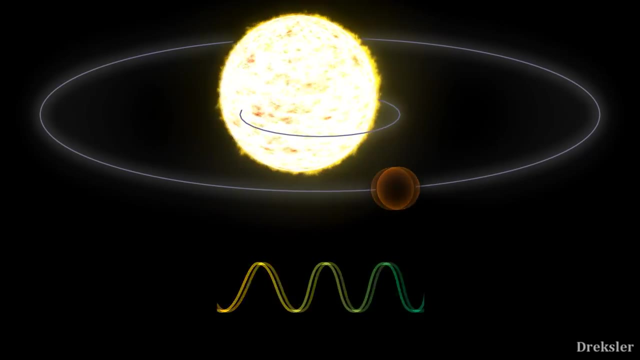 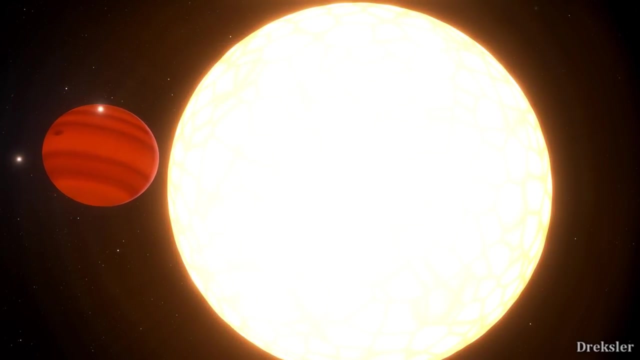 by two methods together. One method needs to give away the mass of the planet, like the wobble method, which gives away the mass of the planet by telling us how much it tugs usually on its host star, And the other method needs to give away the size of the planet. 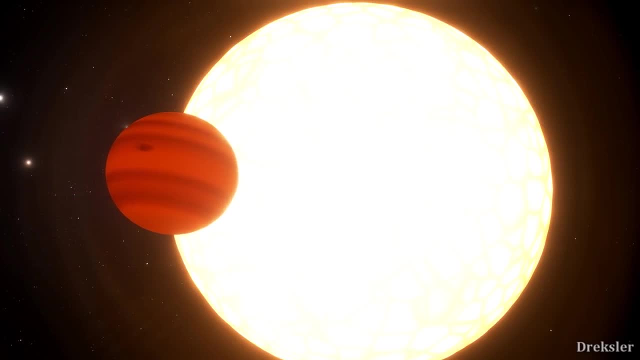 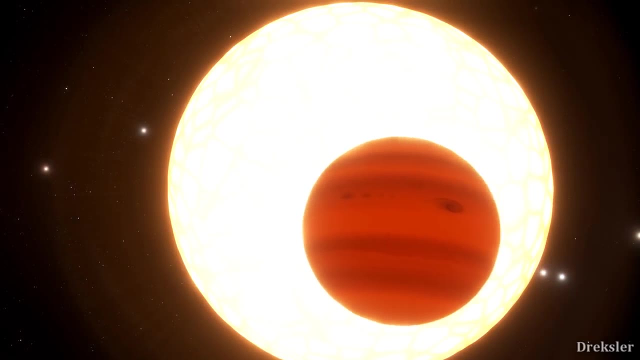 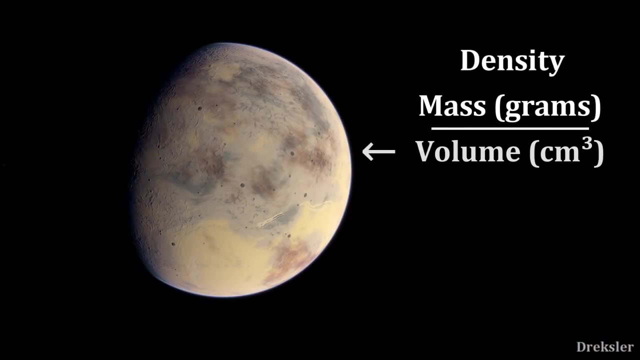 like the transit method, which gives away the size of the planet due to dimming that it causes to its host star as it passes in front of it. So when a planet is detected through both of those methods, since density is just mass divided by volume, then that 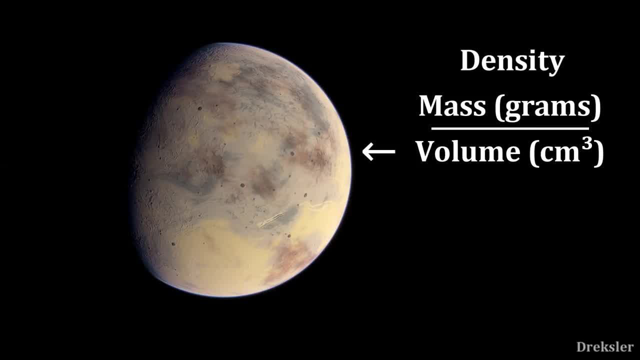 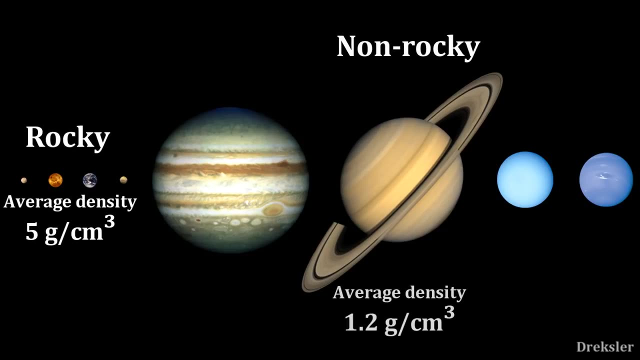 gives away the density of the planet. Density of the planet tells us the likely composition of the planet and that also tells us with some degree of certainty if a planet is to be terrestrial. That is because rocky, terrestrial planets are much denser than non rocky planets. 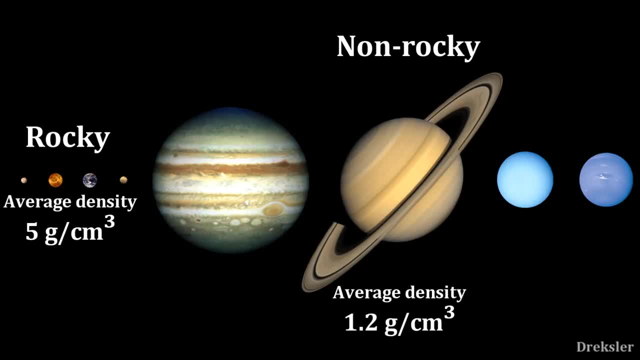 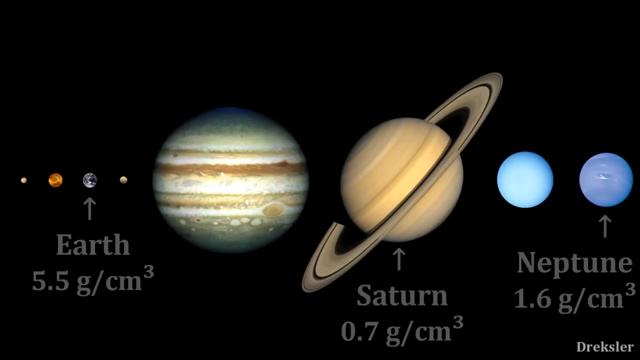 Simply because rocky planets are well made, mostly out of heavy elements — certain rocks. So, for example, the Earth is about 3.5 times denser than Neptune and about 7 times denser than Saturn. Saturn is actually even less dense than water. 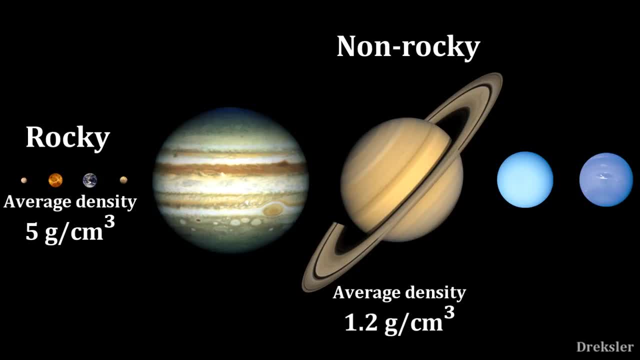 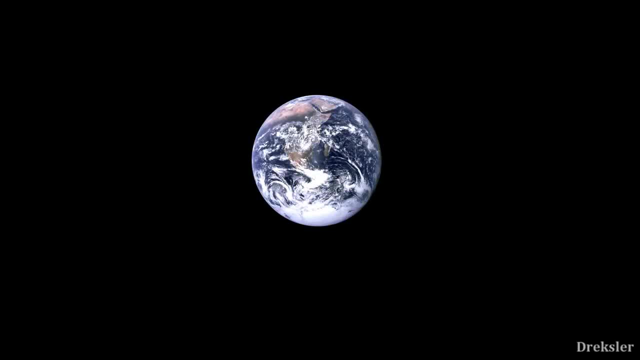 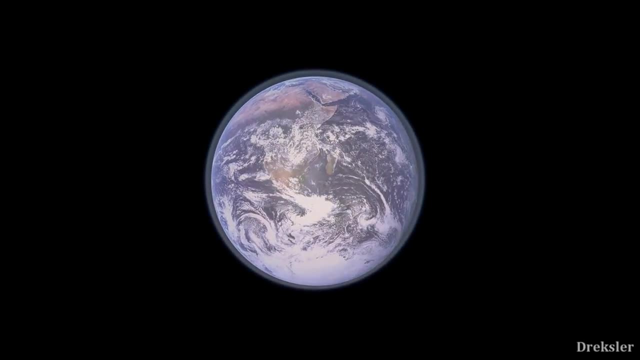 All rocky terrestrial planets in the solar system show that they are denser than all matter non-terrestrial planets. So anyways, study results show us already that usually, as planets grow beyond 1.6 times that of the Earth, they also get lower in density because they have enough mass. 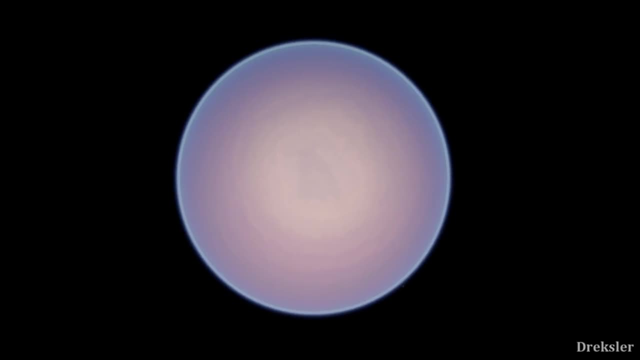 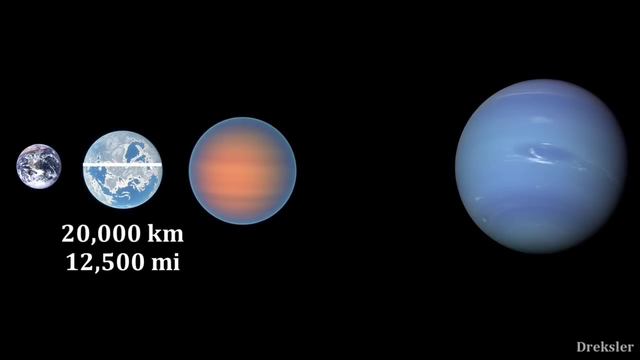 to start capturing light gases, helium and hydrogen. So that means that planets that have a diameter beyond 20,000 kilometers also usually have a density way below the one for certainly rocky terrestrial planets. That is because they are either engulfed in gas, so they are not. 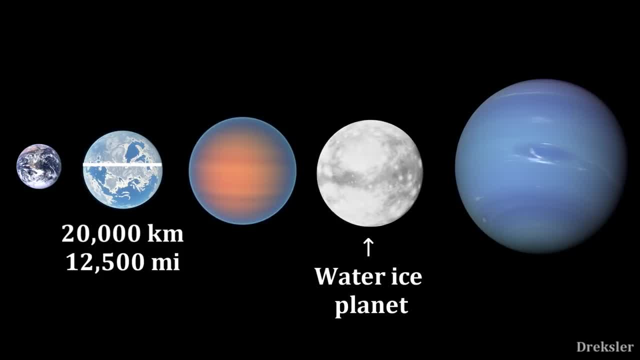 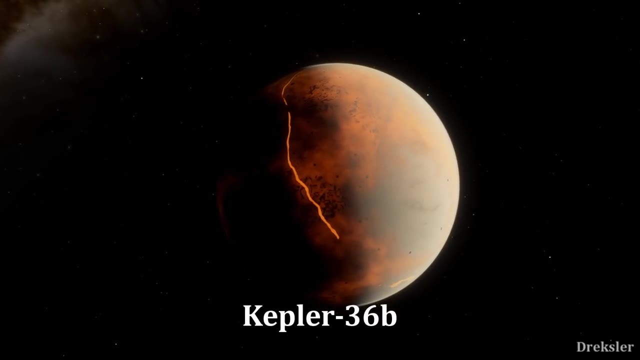 terrestrial, or maybe they are terrestrial, but they are mostly water ice, which is low in density. So the largest rocky terrestrial planets in the universe are about 20,000 kilometers in diameter. For example, Kepler-36b, a planet found in 2012.. It is about 1,750 light-year-old. 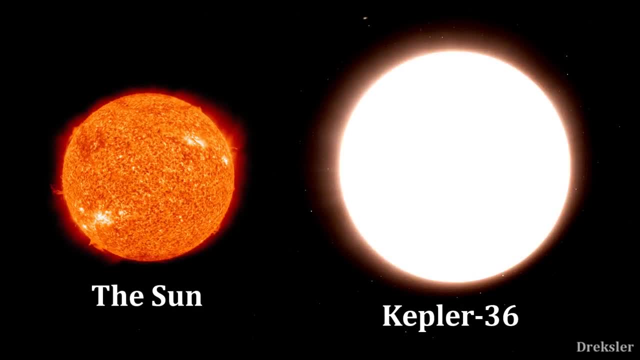 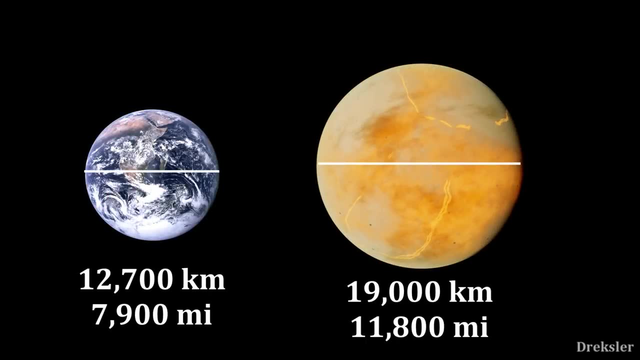 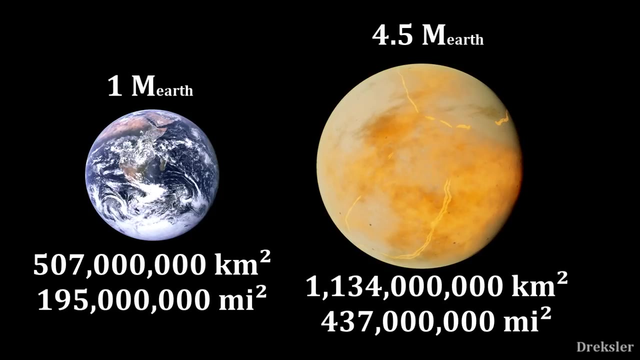 years away from the Earth, and it is orbiting a sub-giant star. It is larger than the Sun. Now, the estimates put the diameter of this planet at about 19,000 kilometers, so its surface area is 2 times greater than the Earth's. Its mass is 4.5 times that of the Earth, meaning 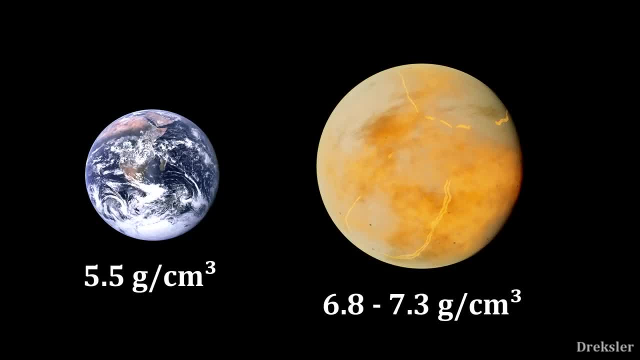 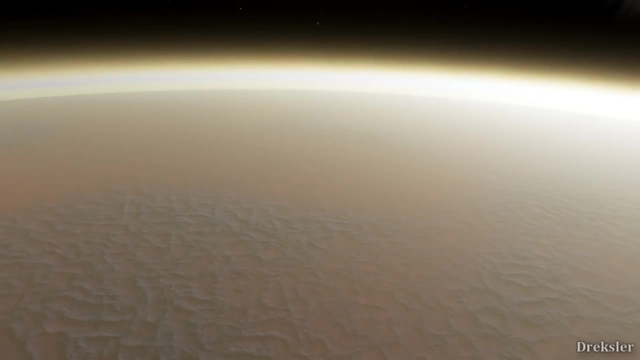 its density is 6.8 grams per centimeter cubic, compared to 5.5 grams per centimeters cubic of Earth. This strongly indicates that this is a terrestrial planet. Also, the surface gravity of this planet is about 2 times greater than the Earth's, so you would be 2 times heavier there. 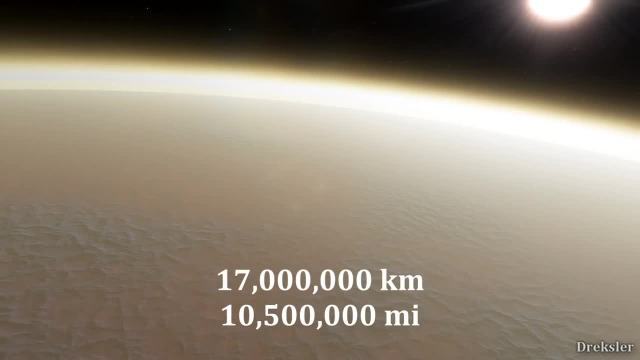 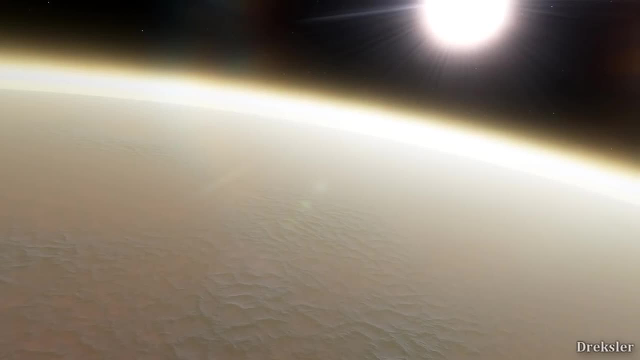 Now Kepler-36b is about 17 million kilometers away from its host sub-giant star, so any hydrogen and helium is quite easily stripped away from its surface because of harsh solar winds, And also the extreme temperature at its surface makes it hard to keep the Earth. 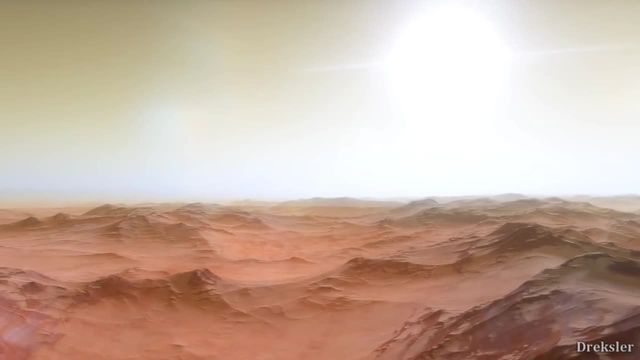 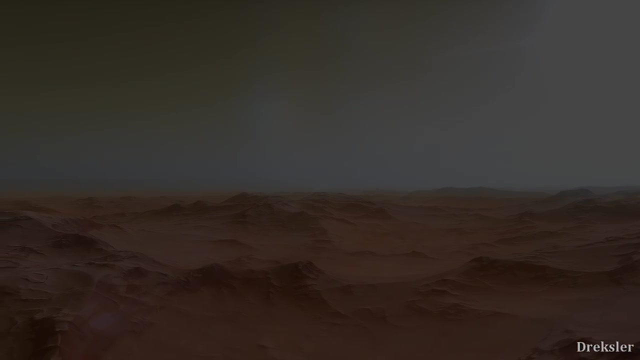 under its control. This is because it is very hard to keep the light, hydrogen and helium with such a surface gravity. But if it had a slightly stronger surface gravity then it would have started capturing hydrogen and helium. So about 20,000 kilometers is near the limit for rocky terrestrial. 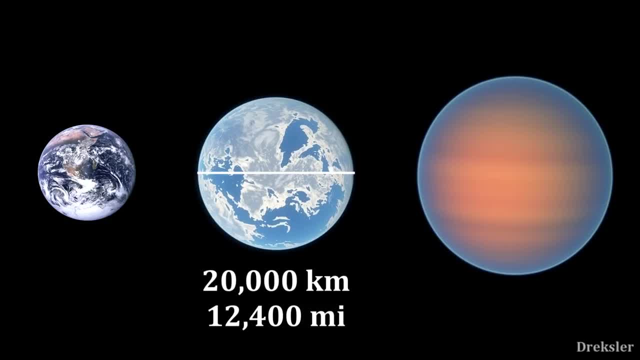 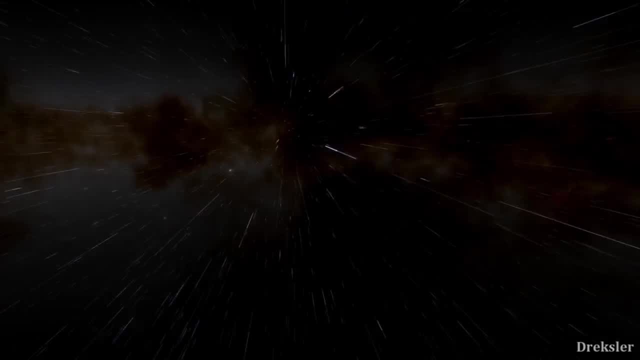 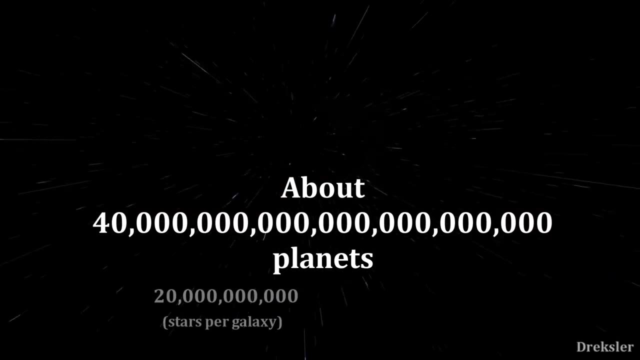 planets Beyond that, they start having too much gravity, which causes hydrogen and helium to be trapped on their surface. Now the number of planets in the observable universe is about 46,000,000,000.. And the total number of planets in the observable universe is about .5 billion, since there 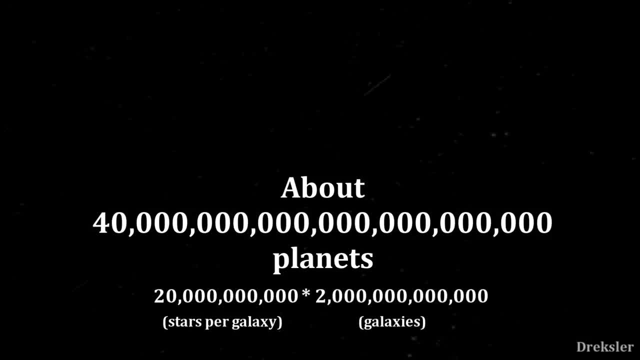 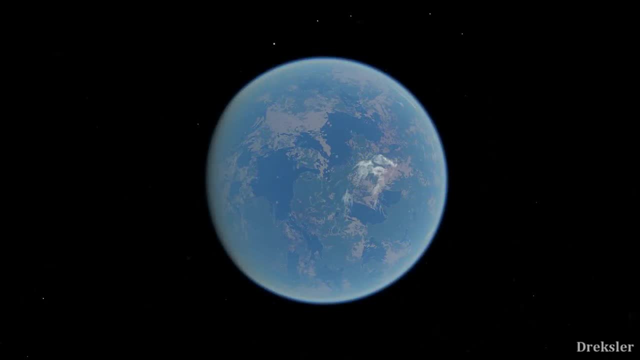 is very approximately about a planet per star and there are about 20 billion stars per galaxy And there are about 2 trillion galaxies in the observable universe. considering that there are likely many planets out there in the universe that are roughly about 20,000. 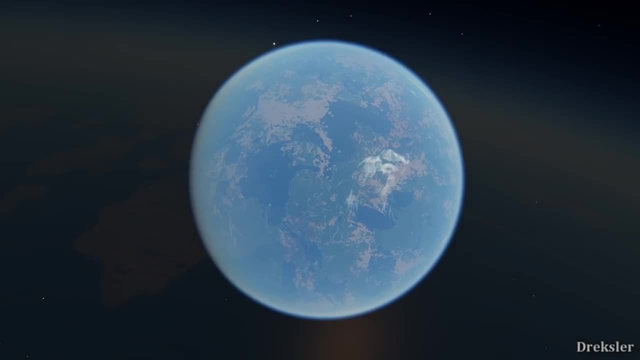 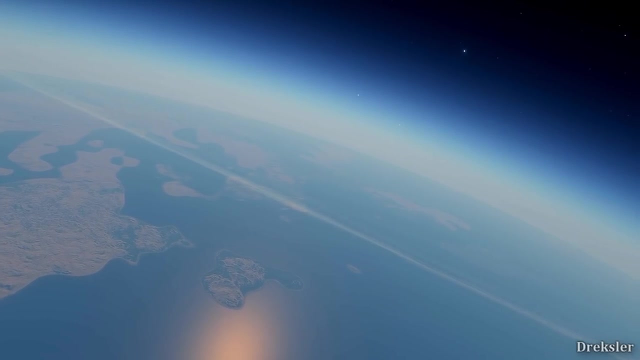 kilometers long, that have a surface gravity around 1.7 times that of the Earth, that have oceans of water on them, But since atmospheres of 7 billion are in the observable universe, Such large rocky planets would likely be much thicker due to a stronger surface gravity. 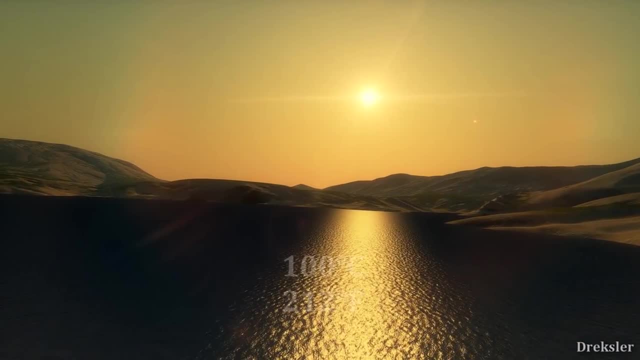 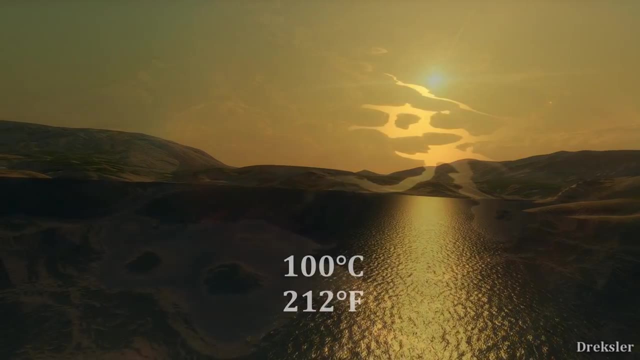 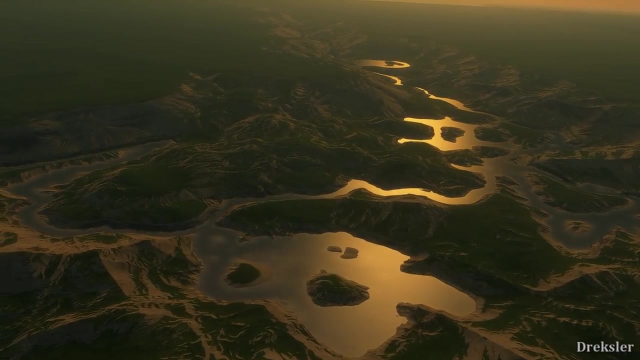 that could allow for oceans of water that are, on average, 100 degrees Celsius hot. That is the boiling point here on Earth at the sea level. But because their atmosphere would usually be thicker, that is not the boiling point on such planets. That is all, because increased pressure increases the boiling point. Some speculations also say that the tectonic activity of 20,000 km long rocky terrestrial planets would likely be usually much greater than that on the Earth, So continental movement on such planets would be happening much quicker compared to Earth. Still, what I talked about there is only rocky terrestrial planets. 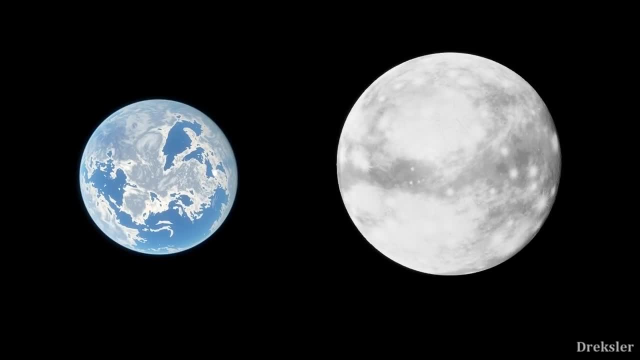 The size limit for water ice terrestrial planets is quite a bit above 20,000 km. That is because water ice is much less dense than rock, So it takes more water in terms of size to get to the point at which the water ice planet. 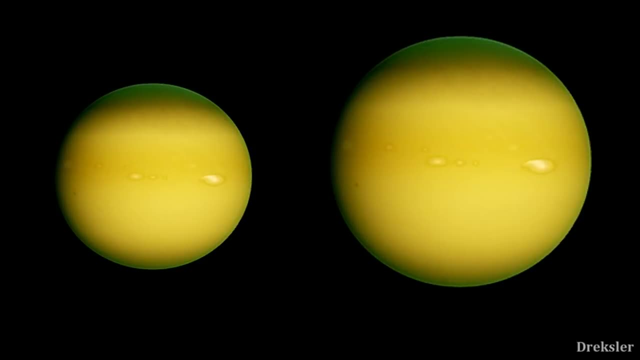 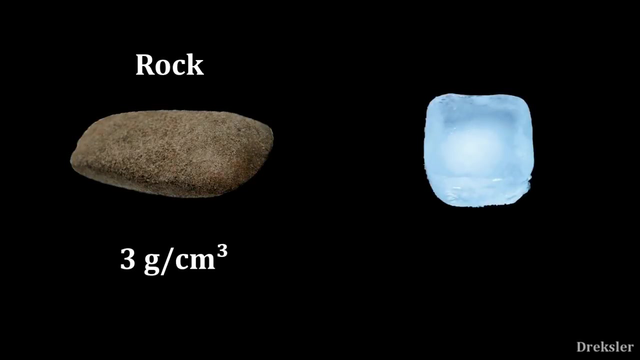 starts having the necessary gravity to start capturing hydrogen and helium. So, for example, the density of rocks on Earth's surface averages roughly around 3 grams per centimeter cubic And the density of water ice is 1 gram per centimeter cubic, So 30 grams of water ice takes up a space of 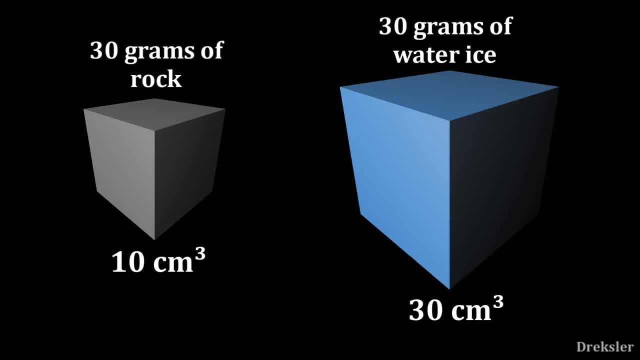 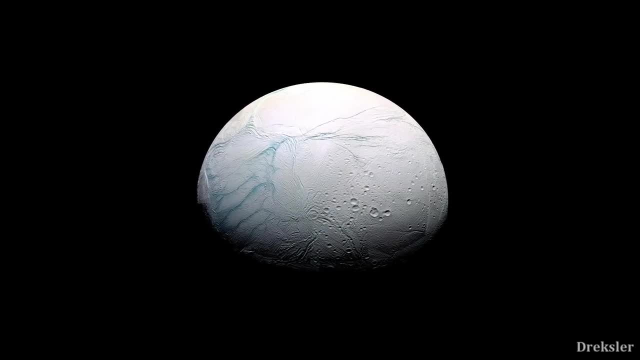 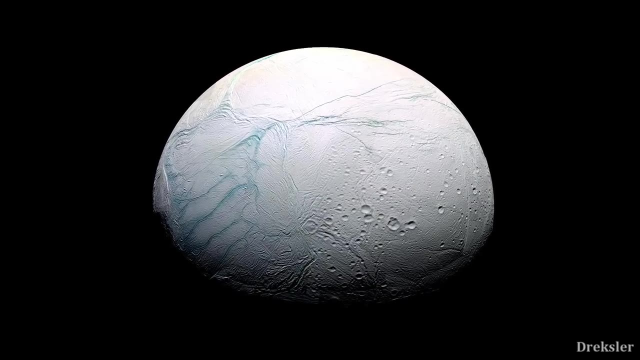 30 centimeters cubic, While 30 grams of rock takes up a space of 10 centimeters cubic. Water is also the third most common molecule in the universe, since it's made out of very common elements, And many moons and planets in the solar system are either a 50-50 mix of water, ice and rock. 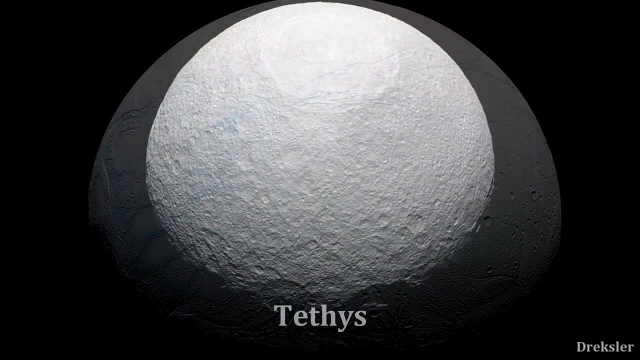 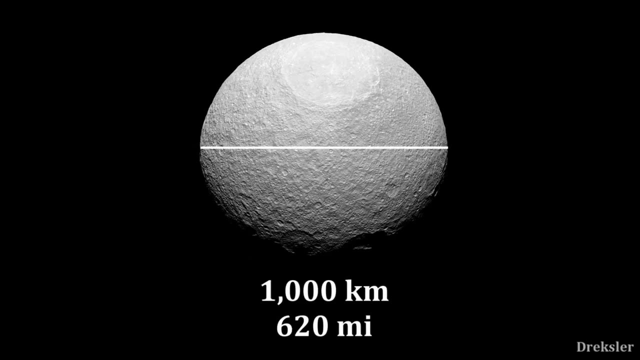 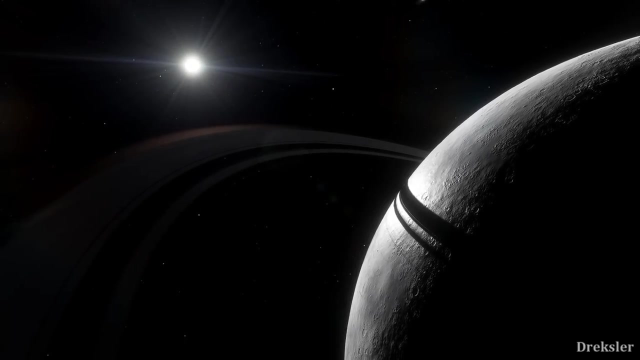 or are mostly water ice. For example, the moon of Saturn, Tethys, has nearly the exact same density as that of water ice, Indicating that this 1,000 kilometer long moon is nearly just pure water ice. So, considering that there are about 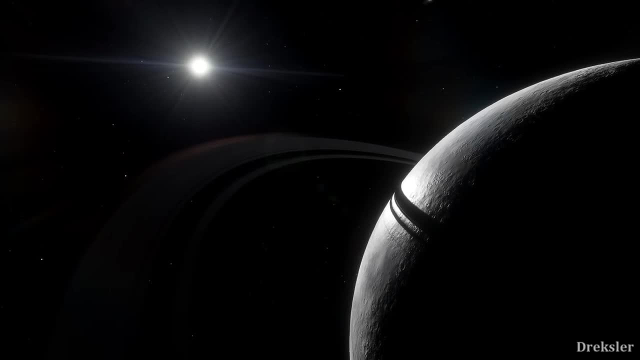 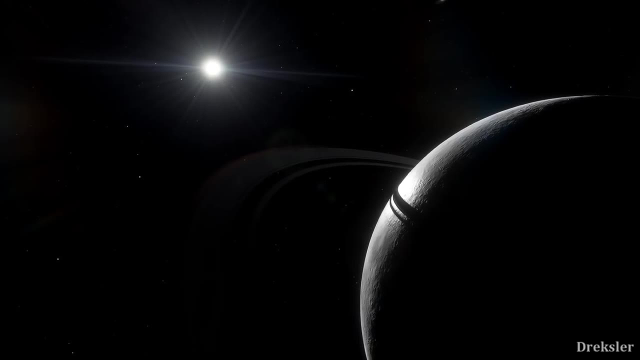 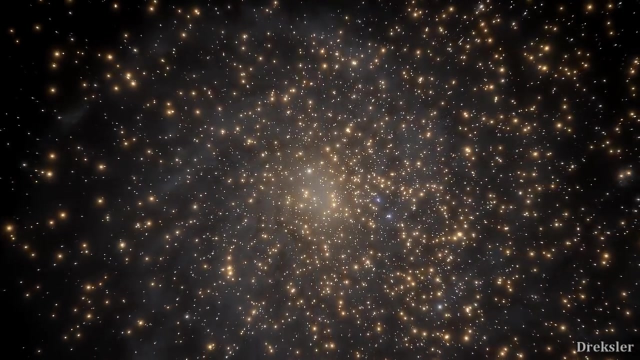 46 billion planets just in the observable universe, and considering that water ice is extremely common, there are quite likely many water ice worlds that have diameters up to about 28,000 kilometers, Now the line in size beyond which water ice planets certainly start capturing hydrogen and helium. 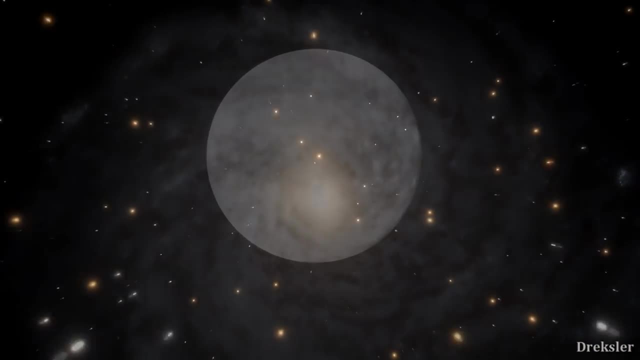 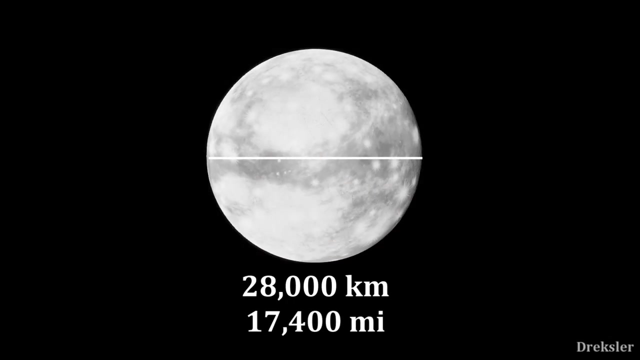 is not as certain as with rocky planets, But a reasonable guess puts it at about 28,000 kilometers. Since very approximately beyond that size the water ice planets generally start having enough mass to start having a surface gravity beyond the one for the Earth. 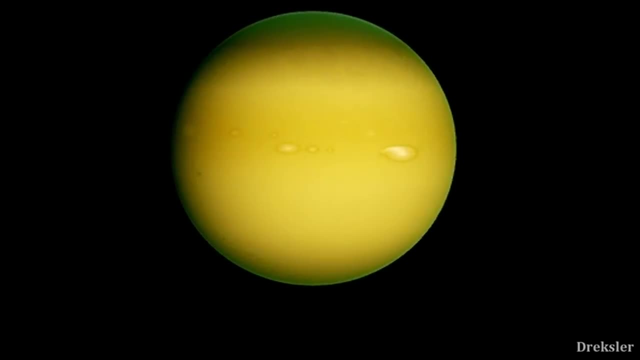 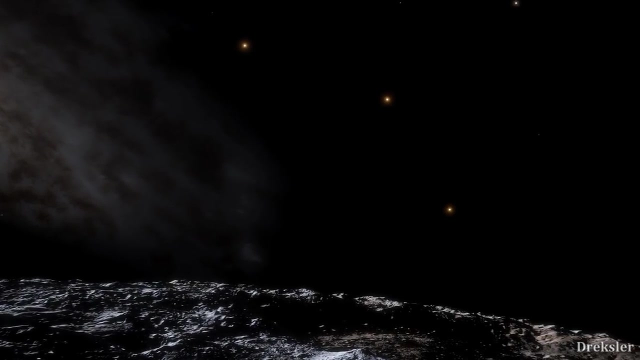 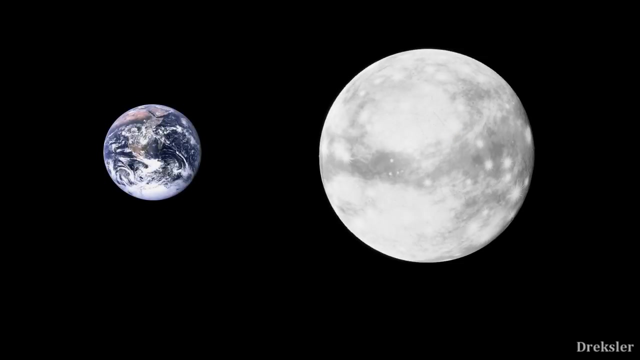 So likely that makes them start capturing hydrogen and helium. So out of many sextillions of planets out there, there likely is a planet with a diameter of 28,000 kilometers. That is nearly entirely water, ice, and this is pretty much near the limit for terrestrial planets overall.